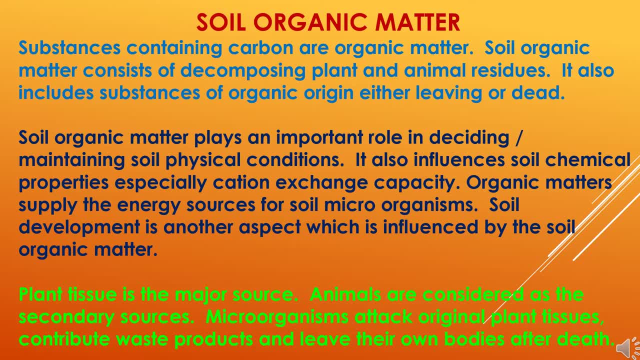 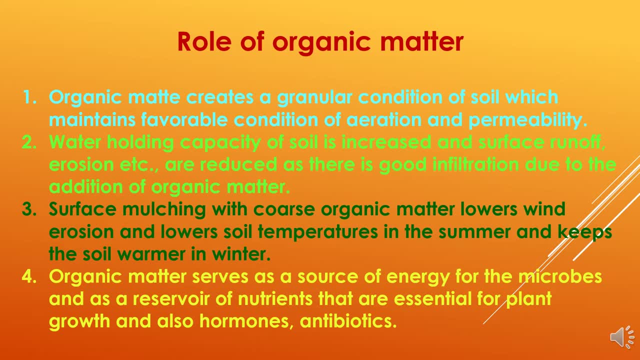 bodies after death and contributing to the soil: organic matter. Now to study role of organic matter. First, organic matter creates a granular condition of soil which maintains favorable condition of aeration and permeability. Second, water holding capacity of soil is increased and surface runoff, erosion etc are reduced as there is good infiltration due to the addition. 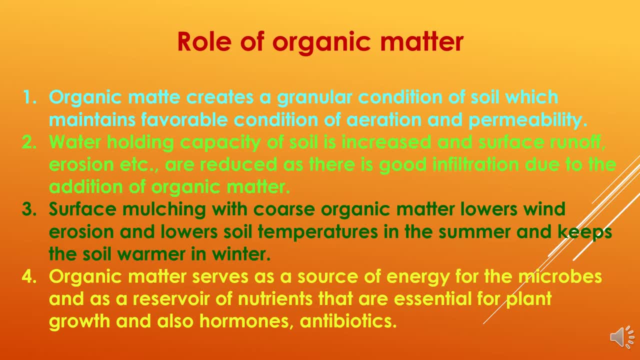 of organic matter. Third, surface mulching with coarse organic matter lowers wind erosion and lowers soil temperatures in the summer and keeps the soil warmer in winter. Fourth, organic matter serves as a source of energy for the microbes and as a reservoir of nutrient and nutrient nutrients that are essential for plant growth, and also hormones and antibiotics. 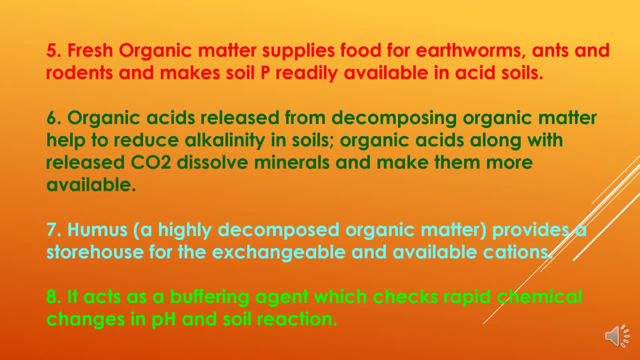 Fifth, fresh organic matter supplies food for earthworms, ants and rodents and makes soil phosphorus readily available in acidic soils. Sixth, organic acids released from decomposing organic matter helps to reduce alkalinity in soils. Organic acids, along with released carbon dioxide, dissolve minerals and make them more available to the plants. 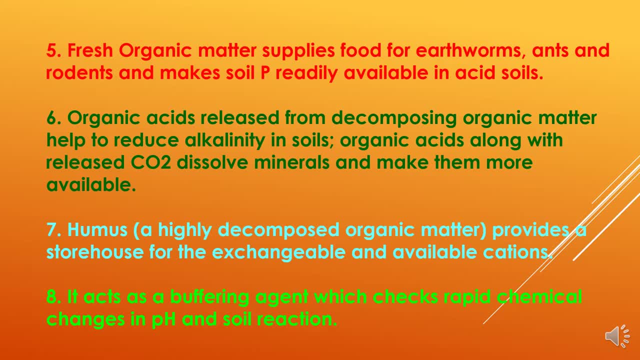 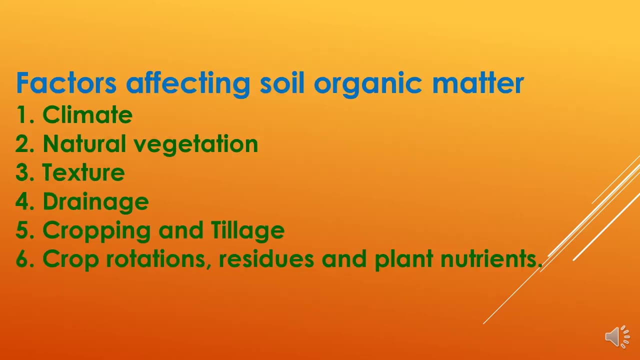 Seventh, humus, which is a highly decomposed organic matter, provides a storehouse for the exchangeable and available cations. Eighth, Soil organic matter X is a buffering agent which checks rapid chemical changes in pH and soil reaction. The factors which are affecting soil organic matter: First one is climate. Second is natural vegetation. Third is soil texture. Fourth, 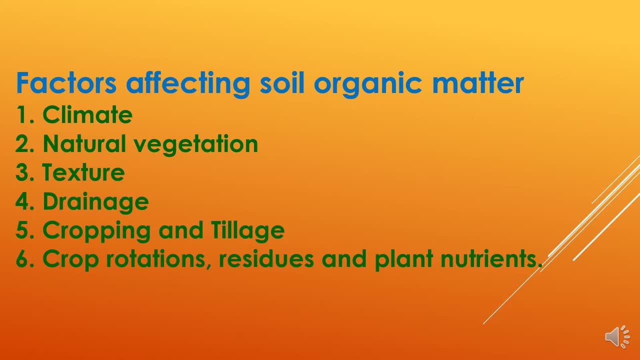 is drainage, Fifth is cropping and tillage. And sixth cropping of soil. Fifth and sixth cropping of soil. Soil organic matter acts as a buffer against soilSoil organic matter acts as a buffer against sixth crop rotations, residue and plant nutrients. Now we will discuss about each topic in details. 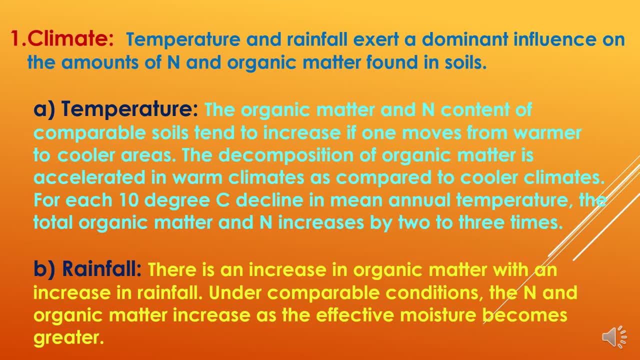 First we will study about climate. Temperature and rainfall exert a dominant influence on the amount of nitrogen and organic matter found in soils. Under climate, there are various parameters which are playing important role for soil organic matter like first, one is temperature. The organic matter and nitrogen content of comparable soils tend to increase if one. 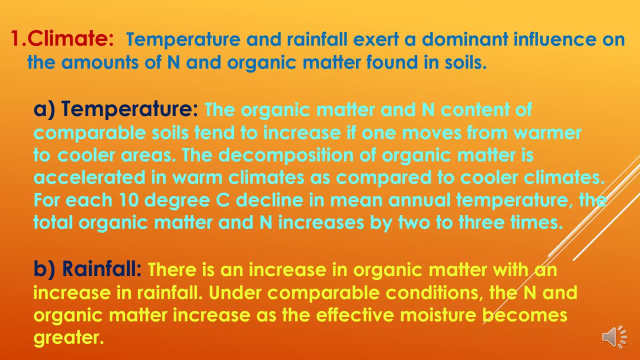 moves from warmer to cooler areas. The decomposition of organic matter is accelerated in warm climates as compared to cooler climates. For each 10 degree Celsius decline in mean annual temperature, the total organic matter and nitrogen increases by two to three times. Second is rainfall. There is 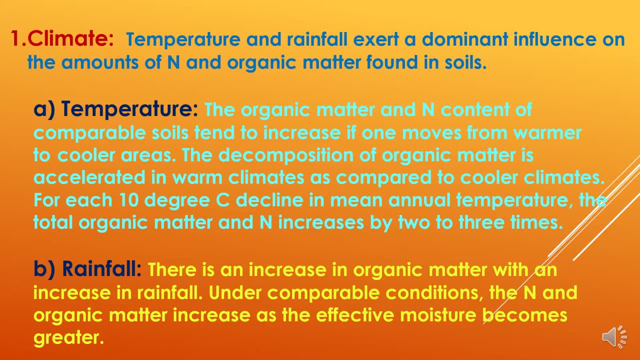 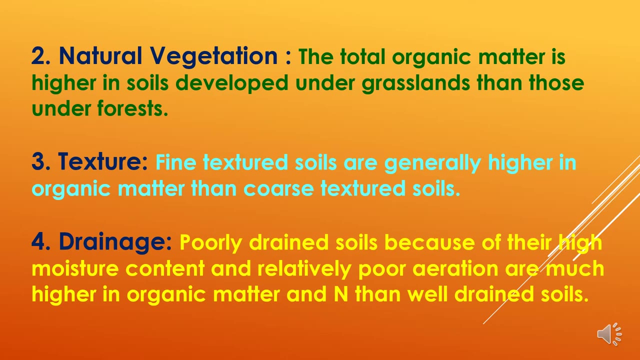 an increase in organic matter with an increase in nitrogen content In the case of organic matter. in rainfall, Under comparable conditions, the nitrogen and organic matter increases as the effective moisture becomes greater. Second factor affecting soil organic matter is natural vegetation. The total organic matter is higher in soils. 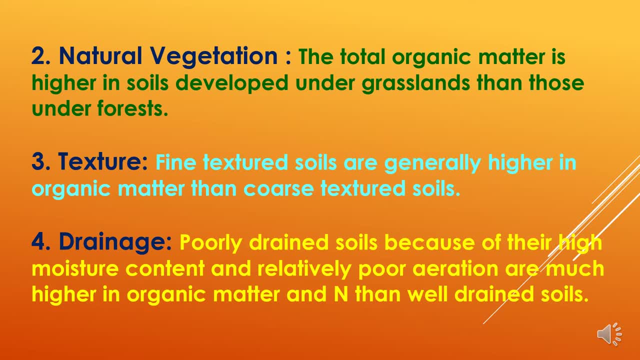 developed under grasslands than those under forests. Third one is texture. Fine texture soils are generally higher in organic matter than coarse texture soils. Fourth is drainage. Poorly drained soils, because of their high moisture content and relatively poor aeration, are much higher in organic matter and nitrogen. 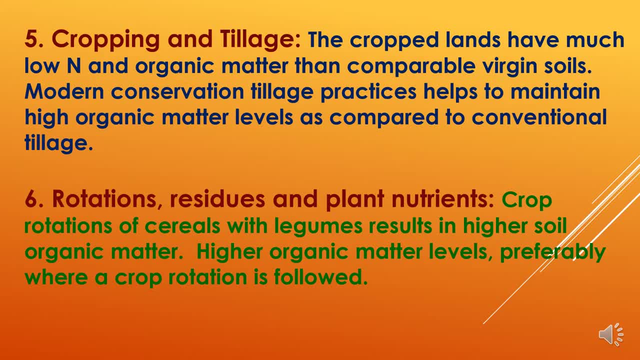 than well-drained soils. Fifth factor is cropping and tillage. The cropped lands have much lower nitrogen and organic matter than comparable virgin soils. Modern conservation tillage practices helps to maintain high organic matter levels as compared to conventional tillage. Sixth is rotations, residues and plant nutrients: Crop rotations of cereals with legumes. 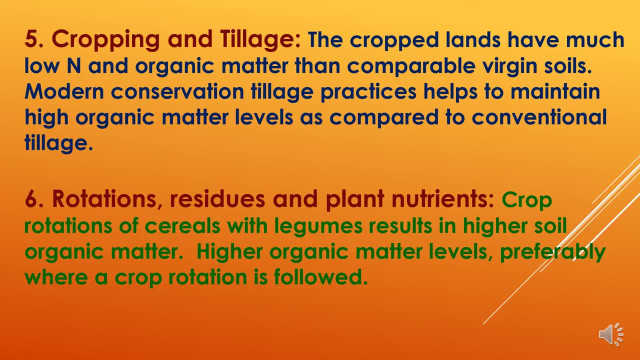 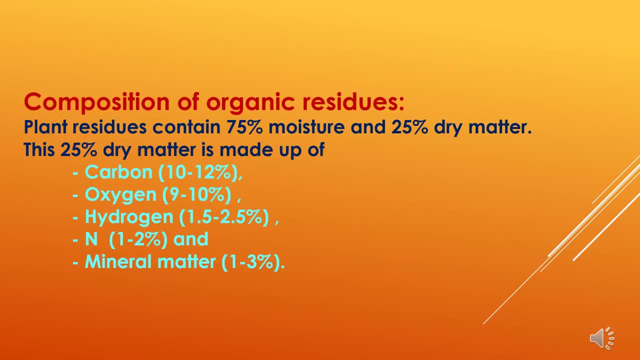 results in higher soil organic matter. Higher organic matter levels, preferably where a crop rotation is followed. Composition of organic residues: Plant residues contain 75% moisture and 25% dry matter, and this 25% dry matter is made up of carbon, 10 to 12 percent oxygen, 9 to 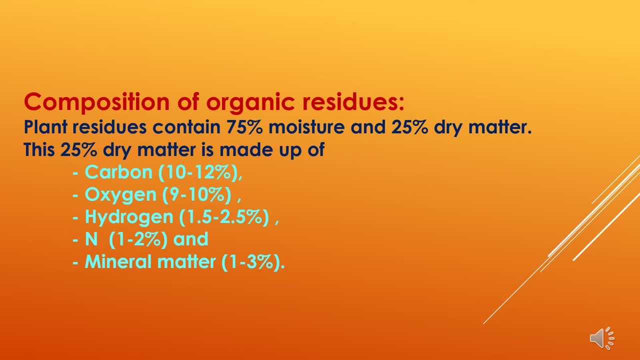 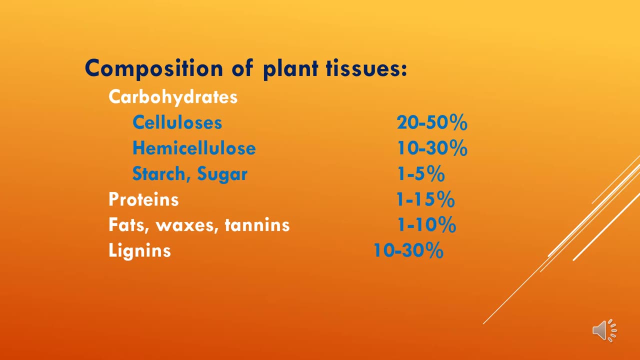 10 percent, hydrogen, 1.5 to 2.5 percent, nitrogen 1 to 2 percent and mineral matter 1 to 3 percent. Here to study composition of plant tissues, There are cellulose having 20 to 50 percent hemicellulose, 10 to 30 percent starch and 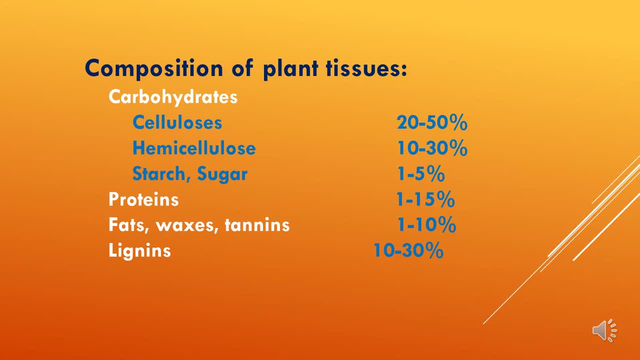 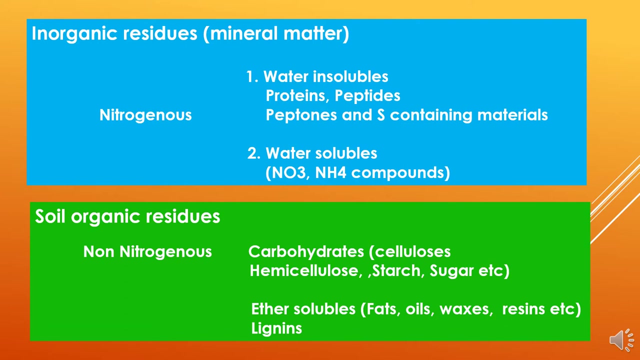 sugar 1 to 5 percent. These three are components of carbohydrates. Then proteins 1 to 15 percent, fats, waxes and tannins 1 to 10 percent and lignins 10 to 30 percent. Here we will study about inorganic residues and soil organic. 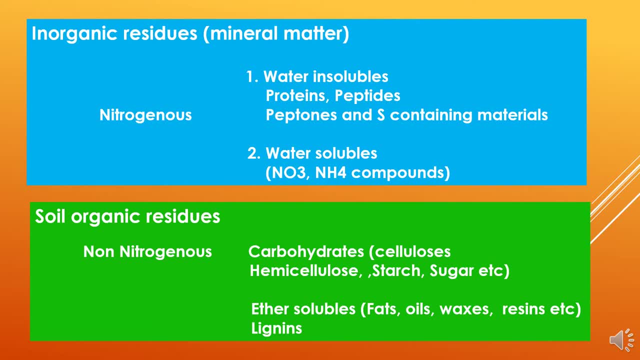 residues. First one is inorganic residue, which is mineral matter. These are the nitrogenous compounds. These are of two types. First one is water insoluble like proteins, peptides, peptones and sulfur containing materials. And second is water solubles like nitrates and 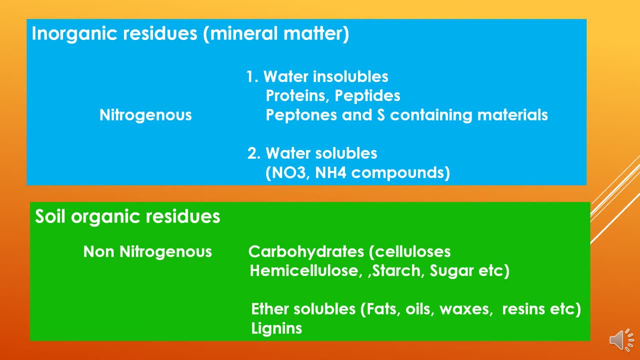 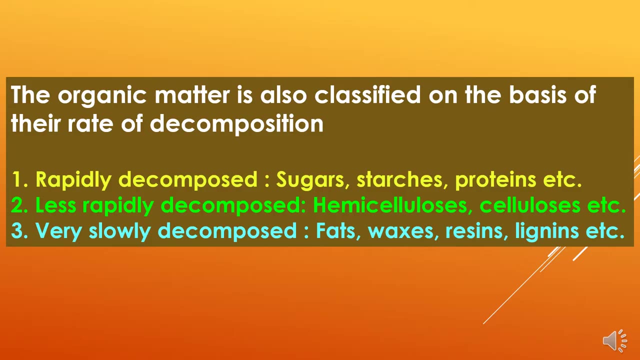 ammonium compounds Under soil organic residues. there are non-nitrogenous and non-sulfuric nitrogenous like carbohydrates, which is containing cellulose, hemicellulose, starch and sugars, And there are some ether solubles like fats, oils, waxes, resins and lignins. 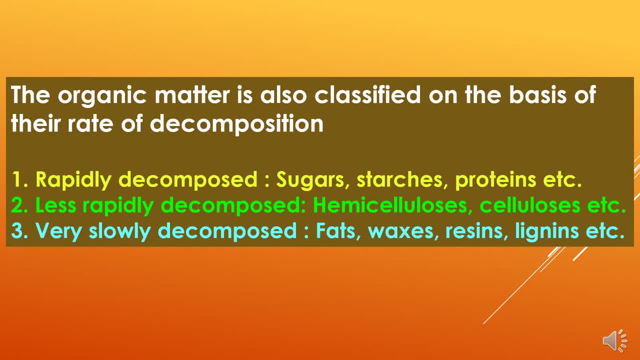 The organic matter is also classified on the basis of their rate of decomposition. Like first, one is rapidly decomposed, under which sugar, starches and proteins are coming. Second is less rapidly decomposed, like hemicellulose and cellulose. And third, very slow decomposed, like fats, waxes, resins and lignins. 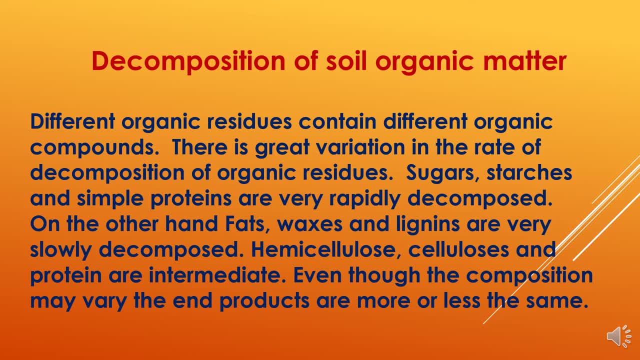 Now to study decomposition of soil organic matter. Different organic residues contain different organic compounds. There is great variation in the rate of decomposition of organic residues. Sugar, starches and simple proteins are very rapidly decomposed. On the other hand, fats, waxes and lignins are very slowly decomposed. 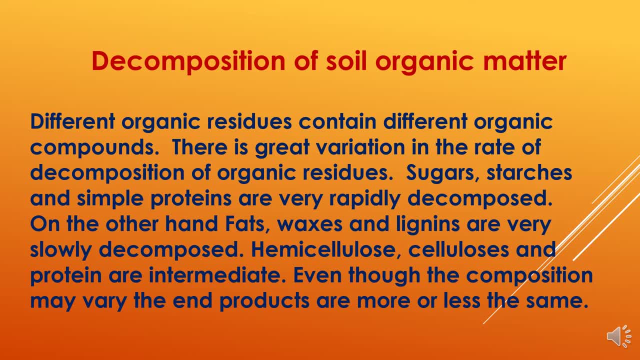 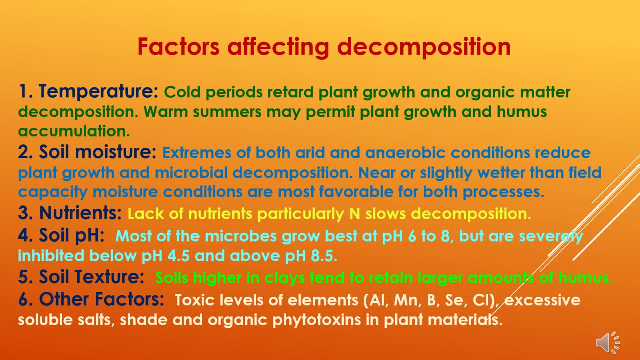 Hemicellulose, cellulose and proteins are intermediate. Even though the composition may vary, the end products are more or less the same. Now to study factors affecting decomposition. First one is temperature. Cold periods retard plant growth and organic matter decomposition. 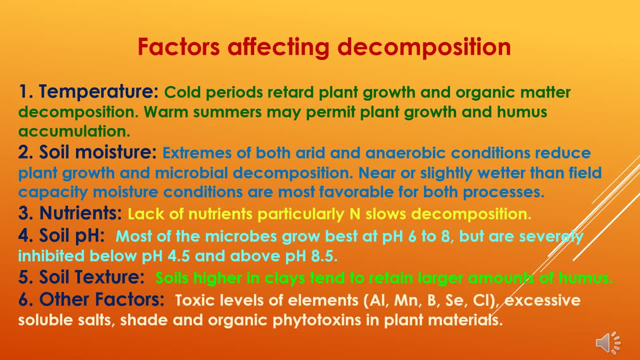 Warm summers may permit plant growth and humus accumulation. Second, soil moisture Extremes of both arid and anaerobic conditions reduce plant growth And microbial decomposition. Near or slightly wetter than field capacity moisture conditions are most favorable for both processes. 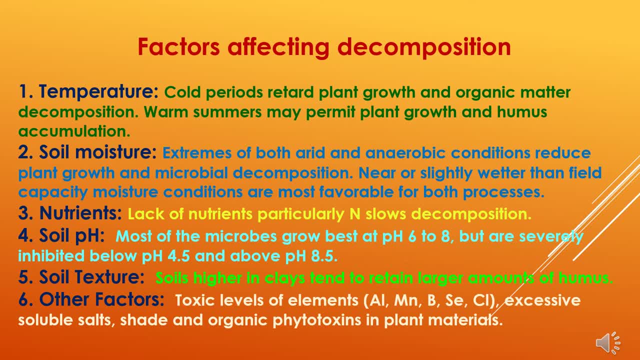 Third is nutrients. Lack of nutrients, particularly nitrogen, slows decomposition. Fourth is soil pH. Most of the microbes grow best at pH 6 to 8, but are severely inhibited below 4.5 and above 8.5.. Fifth is soil texture. 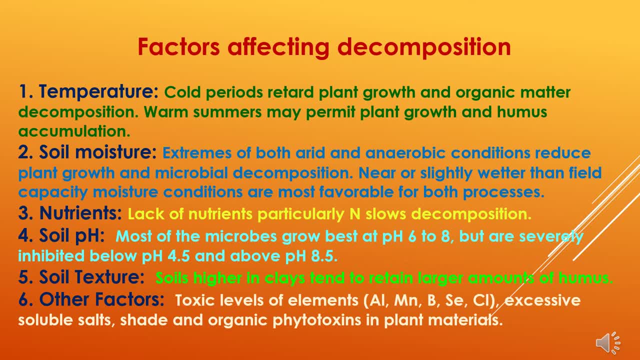 Soils higher in clays tend to retain larger emersion. Soils higher in clays tend to retain larger emersion. Soils higher in clays tend to retain larger emersion. Sixth, other factors like whichислose and aominium*** Aegmaphan nitrogenshade. 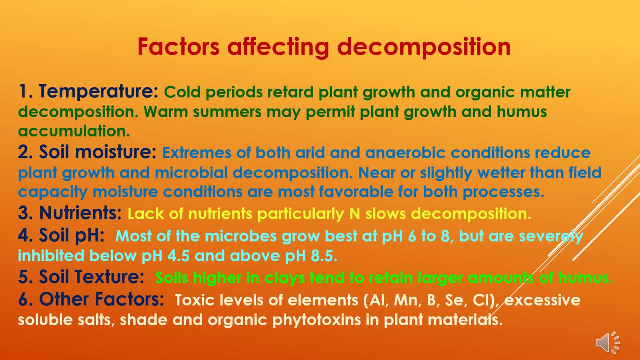 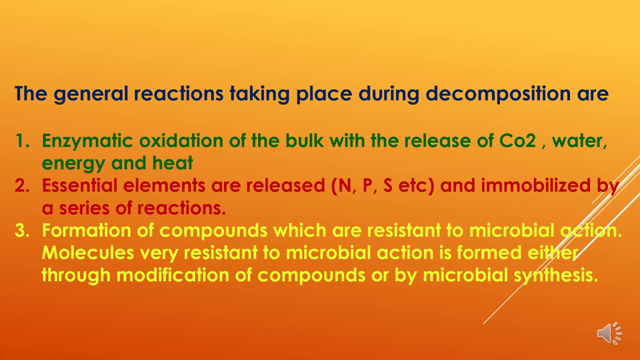 Sixth, other factors like whichsilose and aominium***entre只 kroeg snag Cho casao like toxic-level elements, aluminum. Question about oxygen and magnesium, the general reactions our getting in the human being, the formation that I require. 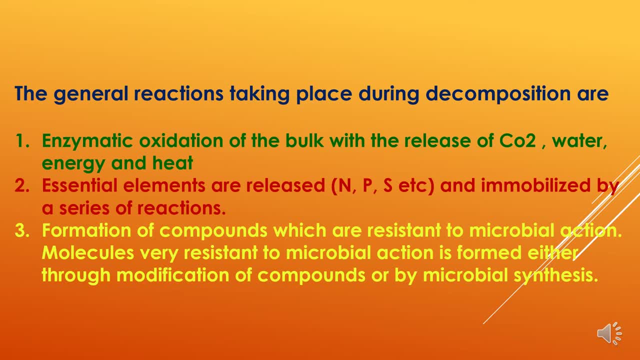 level by which the acid is eliminated. 2. Essential elements are released, like nitrogen, phosphorus, sulfur, etc. and immobilized by a series of reactions. 3. Formation of compounds which are resistant to microbial actions- Molecules are very resistant to microbial actions- is formed either through modification. 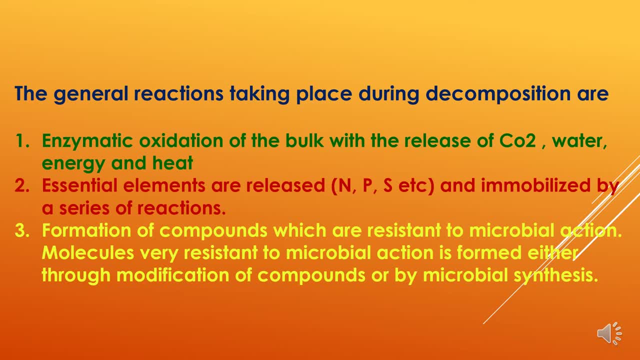 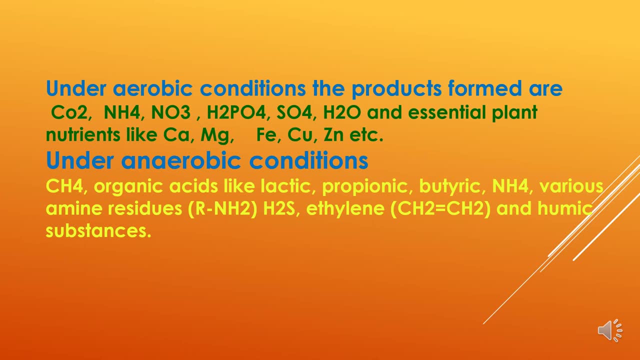 of compounds or by microbial synthesis Under aerobic conditions. the products of decompositions are formed as carbon dioxide, ammonium nitrate, H2PO4,, sulfate and water, and essential plant nutrients like calcium, magnesium, iron, copper, zinc. 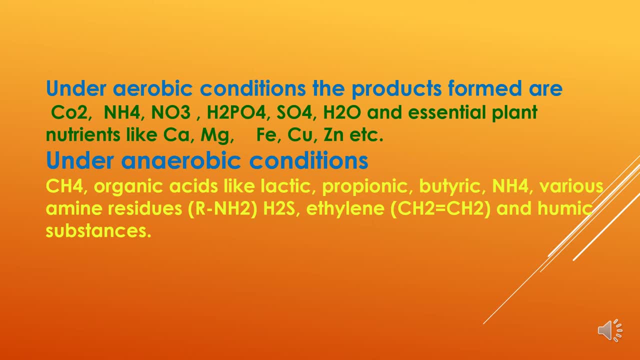 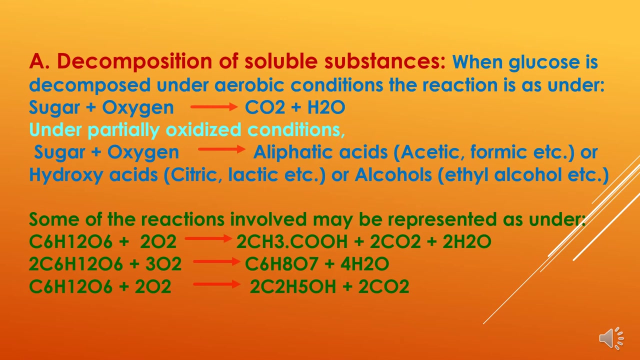 Under anaerobic conditions like methane, organic acids like lactic acid, propionic acid, butyric acid, ammonium, various amine residues, H2S, ethylene, etc. and humic substances. Now to study the decomposition of soluble substances. 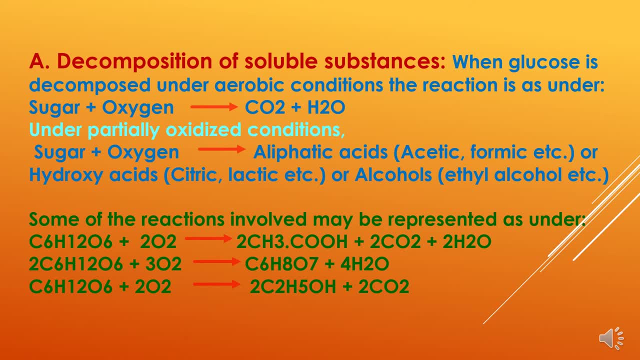 When glucose is decomposed under aerobic conditions, the reaction is found as sugar plus oxygen is equal to carbon dioxide plus water. Under partially oxidized conditions, sugar plus oxygen results into aliphatic acids like acetic and formic acids, or hydroxy acids like citric acid, lactic acid or alcohols. 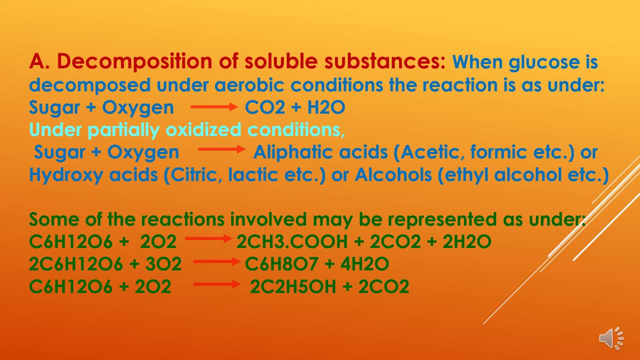 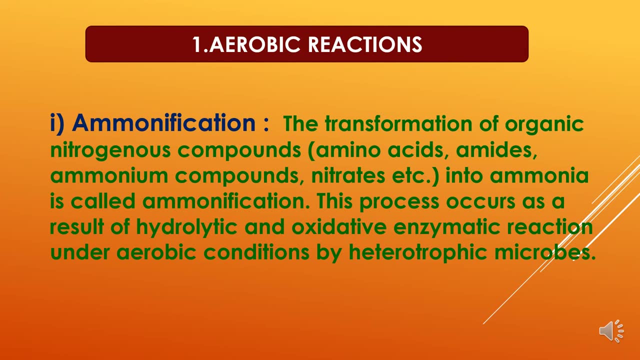 Some of the reactions which are involved may be represented in different way, which are presented here. What is ammonification? The transformation of organic nitrogenous compounds like amino acids, amides, ammonium compounds, nitrates, etc. into ammonia is called ammonification. 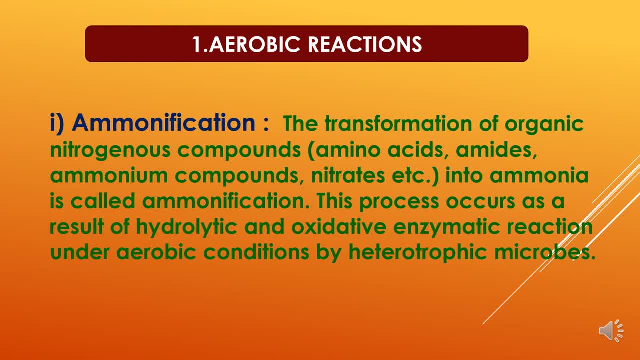 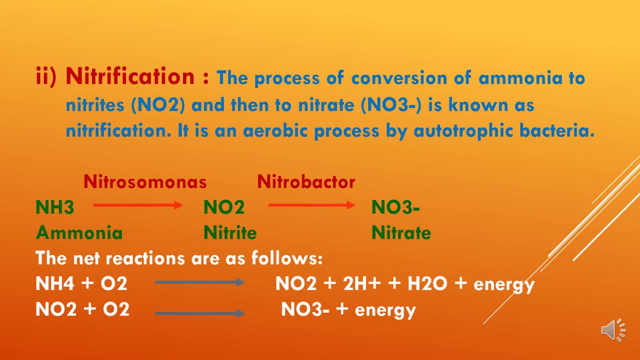 This process occurs as a result of hydrolytic and oxidative enzymatic reactions under aerobic conditions by heterotrophic microbes. Then nitrification: The processes of conversion of ammonia to nitrite NO2, then to nitrite NO3 is known as nitrification. 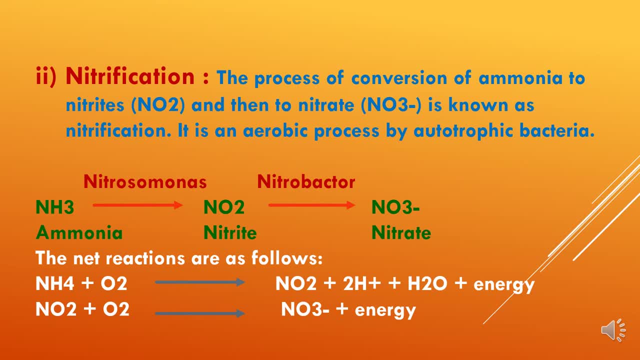 It is an aerobic process by autotrophic bacteria. Here ammonia is converted to nitrite by nitrosomonas bacteria and then nitrite is converted to nitrate by nitrobacteres. The net reactions Which are taking place, like NH4 plus oxygen is equal to NO2 plus 2H plus H2O plus energy. 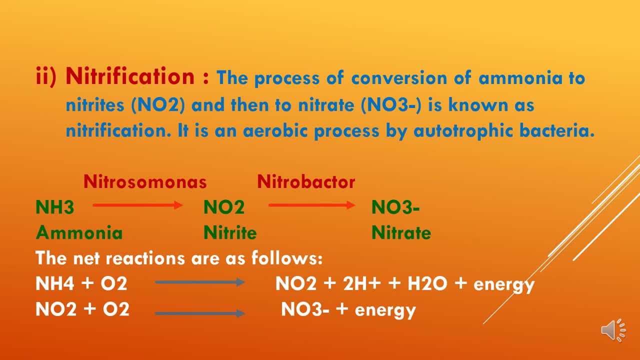 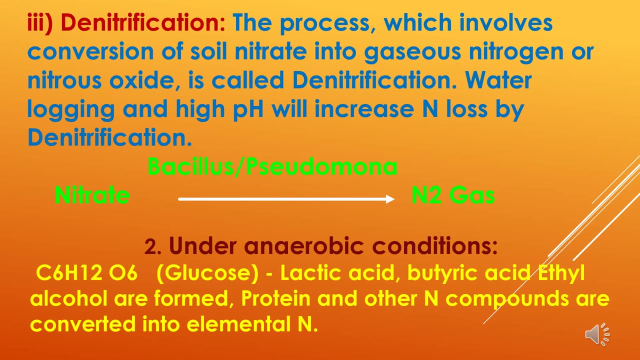 And again when the nitrite is converting to nitrate, NO2 plus oxygen converted to nitrite plus energy. So there are two bacteria which are taking place, Natrosomonas and nitrobacter. Denitrification- The processes which involves conversion of soil nitrate into gaseous nitrogen or nitrification. 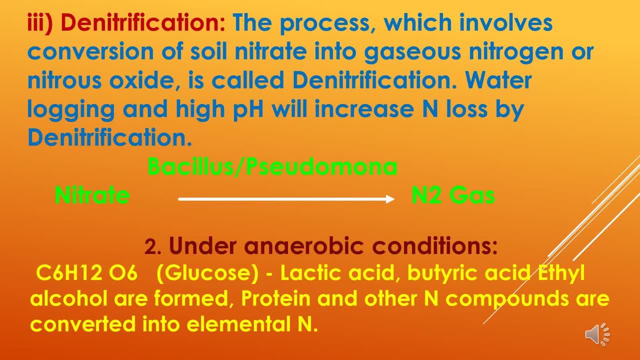 So this process is known as denitrification of the nitrate. So here you can see the process, or nitrous oxide is called denitrification. water logging and high ph will increase nitrogen loss by denitrification and this is taking place by the bacillus and pseudomonas bacteria. 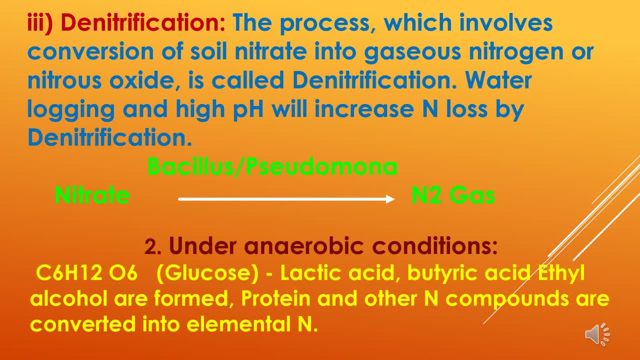 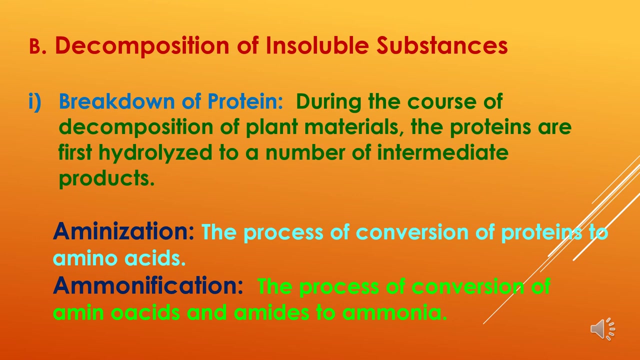 which are converting nitrate to nitrogen gas. and second, reactions are under anaerobic conditions. here the glucose, lactic acid, butyric acid, ethyl alcohol are formed, protein and other nitrogen compounds which are converted into elemental nitrogen. now we'll study the decomposition of insoluble substances. first, breakdown of protein during the course of decomposition of plant. 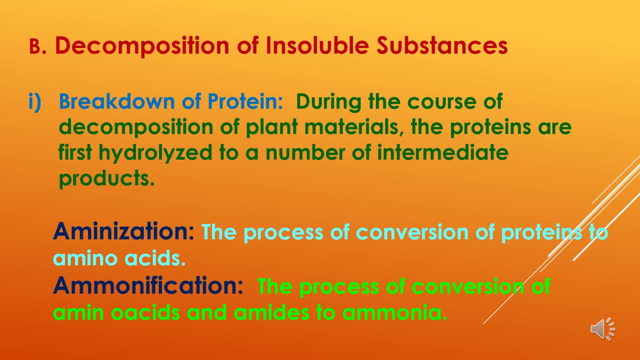 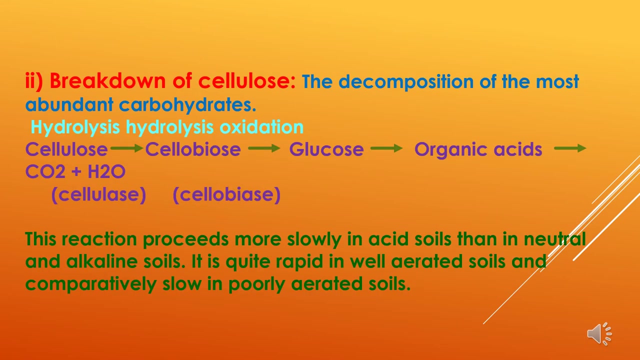 materials, the proteins, are first hydrolyzed to a number of intermediate products. the process like immunization, the process of conversion of proteins to amino acids, then ammonification, the processes of conversion of amino acids and amides to ammonia. second is breakdown of cellulose, the decomposition of the 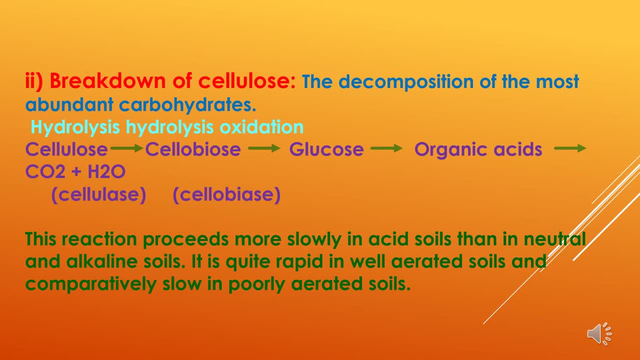 most abundant carbohydrate is cellulose. here the cellulose is converted to cellobiose, then it is converted to glucose, then organic acids and finally breakdown to carbon dioxide and water. this reaction proceeds more slowly in acidic soils than in neutral and alkaline soils. it is 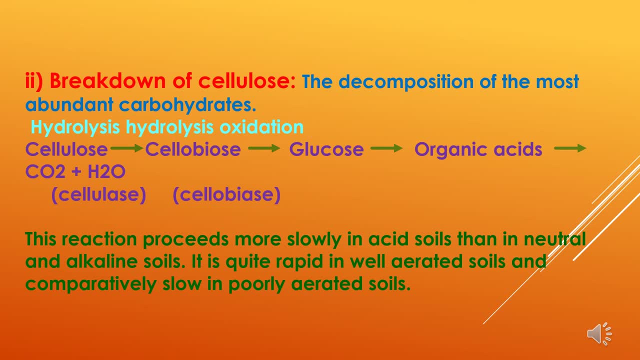 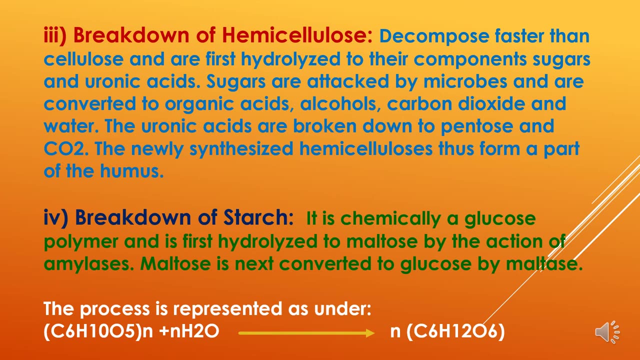 quite rapid in well aerated soils and comparatively slow in poorly aerated soils. now, third breakdown: of hemicellulose decompose faster than cellulose and are first hydrolyzed to their components: sugar and uronic acids. sugars are attacked by microbes and are converted to organic acids, alcohols, carbon dioxide and water. the 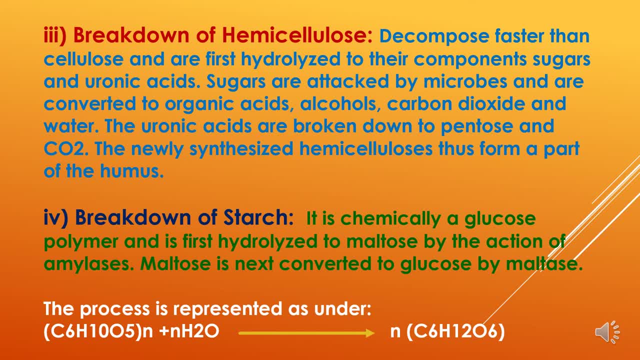 uronic acids are broken down to pentose and carbon dioxide. the newly synthesized hemicellulose thus form a part of the soil, which is called the celulose cellulose, which is very sensitive, and of the humus. Fourth is breakdown of starch. It is chemically a glucose polymer and is first 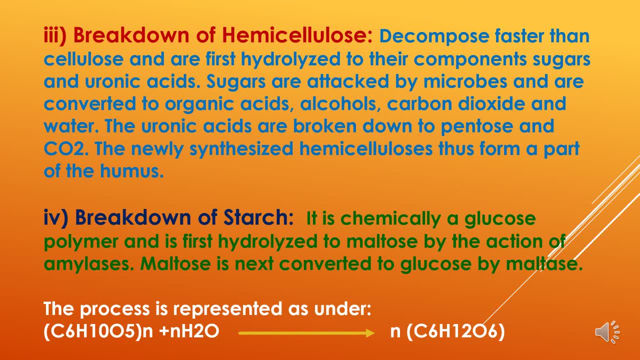 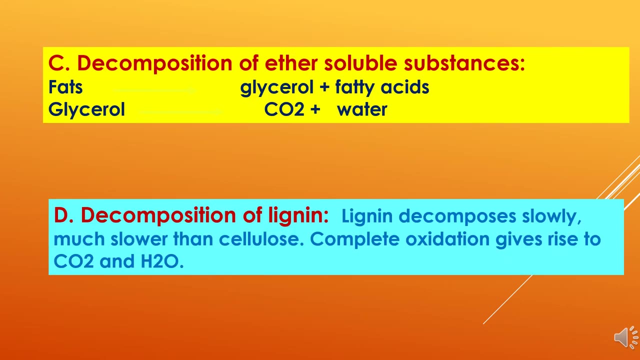 hydrolyzed to maltose by the action of amylase. Maltose is next converted to glucose by maltage. The process is represented like C6H10O5N plus NH2O to NC6H12O6.. Now to study about decomposition of ether soluble substances. Lactphite is after decomposition. 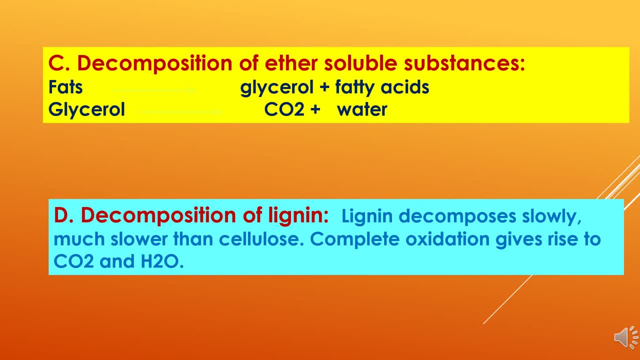 converts to glycerol and fatty acids. Then glycerol is converted to carbon dioxide and water. Then decomposition of lignin: Lignin decomposes slowly, much lower than cellulose. Complete oxidation gives rise to carbon dioxide and water. Now decomposition of sulfur, containing organic 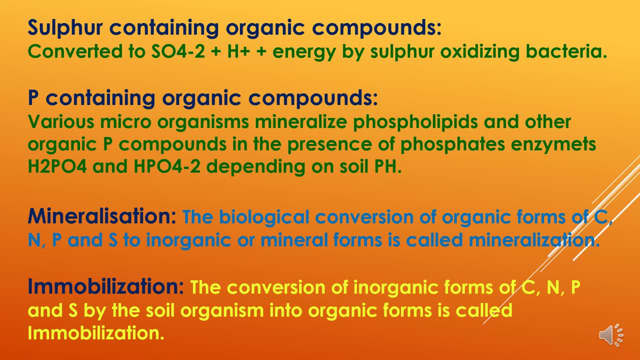 compounds. These are converted to sulfates plus hydrogen, plus energy by sulfur oxidizing bacteria, Then phosphorus containing organic compounds. Various microorganisms mineralize phospholipids and other organic phosphoric compounds in the presence of phosphate enzimates, H2PO4 and H2PO4-2. 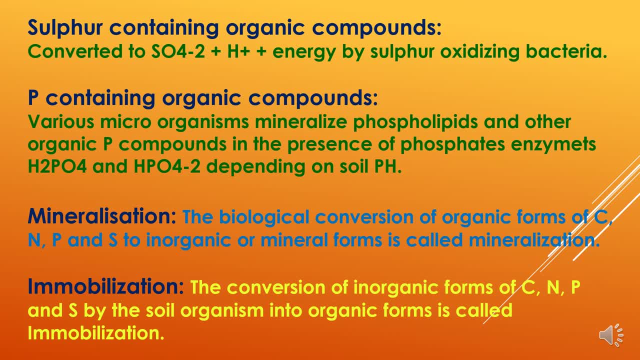 depending on soil pH. What is mineralization? The biological conversion of organic forms of carbon, nitrogen, phosphorus and sulfur to inorganic or mineral form is called mineralization. Then, what is immobilization? The conversion of inorganic forms of carbon, nitrogen, phosphorus?